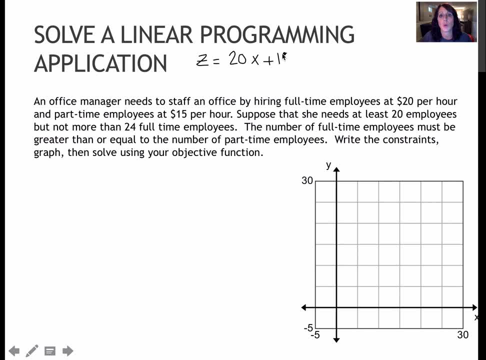 20x plus 15y. So same objective function. we just did on our last question, our last video. If you didn't watch the last video, remember we're looking for, you know, $20 per hour for part-time and 15 per hour for full-time, And the z would be representing the cost. Now these other parts. 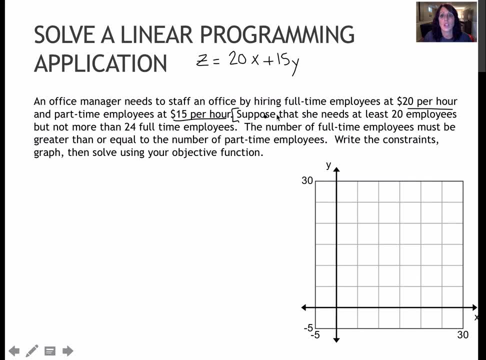 we didn't talk about in the other question. So pay attention to these. She needs at least 20 employees, which means if x is the you know employees, we've got x plus y. at least 20 employees Has to be greater than or equal to 20.. So 20 or more employees, That's one of our constraints. 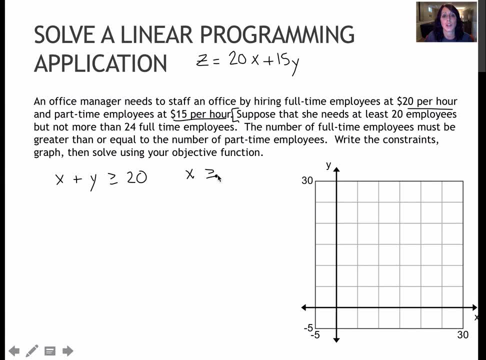 The constraints that are easy that a lot of people forget. X has to be greater than or equal to 0.. Y has to be greater than or equal to 0.. You can't have a negative amount of employees. Cannot have more than 24 full-time employees. So full-time was the x, So x has to be less. 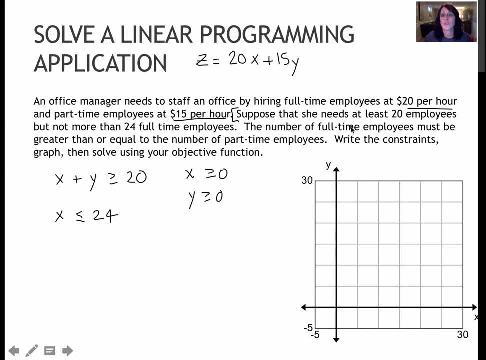 than or equal to 24.. The number of full-time employees must be greater than or equal to the number of part-time employees. So full-time greater than or equal to the number of part-time. Write the constraints graph, solve, etc. So we haven't done any of this last part where we solve. 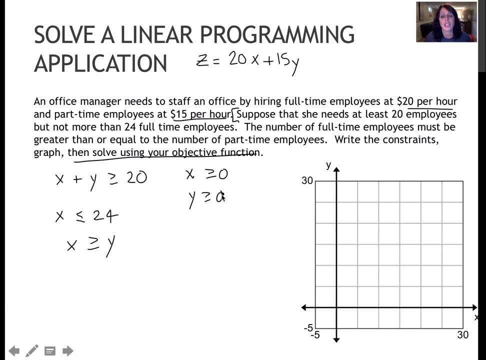 but we should go ahead and be able to graph this. These two are fairly easy. As you can see. I've only given you the graphs for the first quadrant anyway, which means nothing over here will be shaded. Nothing over here will be shaded. 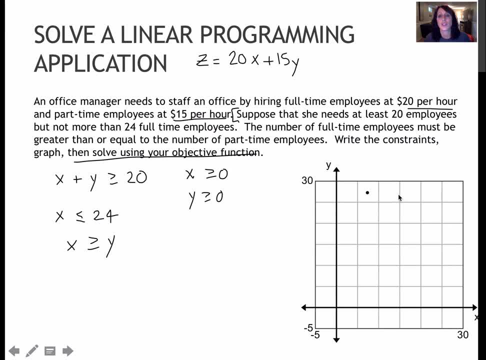 So I would have a line like this, and I have a line like this, and so far it's shaded in this box. Let's look at these: X plus y is greater than or equal to 20.. Obviously, here we're going by fives. 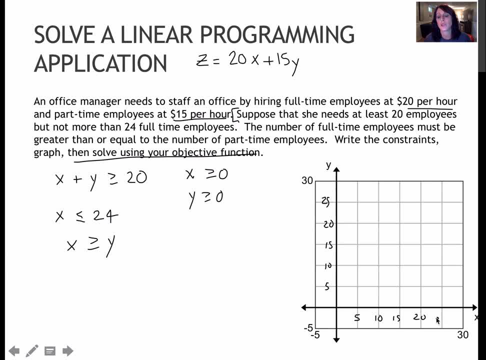 Same thing here: 5,, 10,, 15,, 20,, 25,, 30.. So x plus y equals 20.. I would have a point here at 20 and a point here at 20 using that cover-up trick. 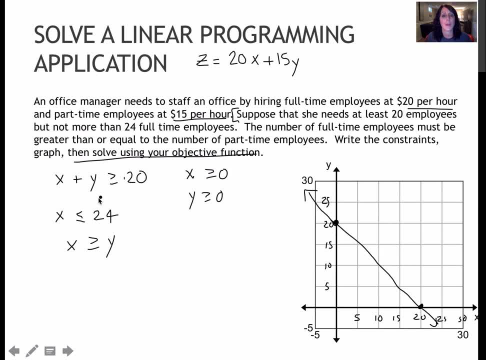 Nice Straight line. I'm not going to worry about shading. yet X is less than or equal to 24.. So x is less than or equal to 24 would be over here. This one, probably not really going to make much of a difference, because that's saying it's to this side. 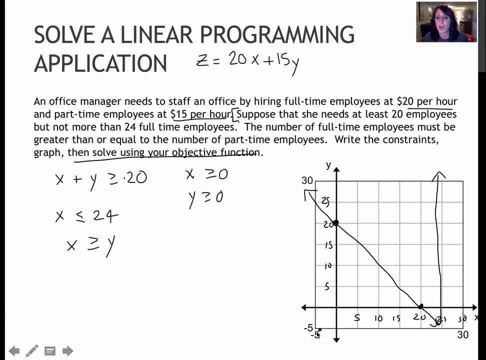 X is greater than or equal to y. X equals y- would be this line right here And now I have to shade, So I know that it's obviously one of these regions. This one, x is less than or equal to 24, would be shaded in this direction. 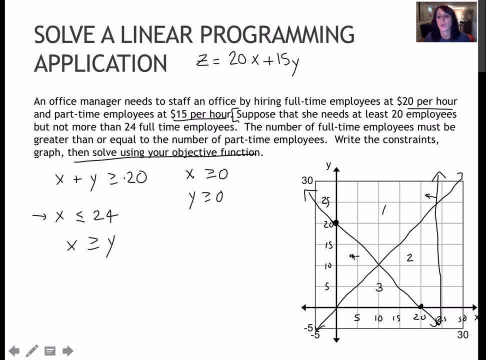 So I'm really looking at 1,, 2,, 3, or 4.. Nothing over here Plug in a test point. So for this one, obviously 0, 0 is a great test point. 0 plus 0 is greater than or equal to 20.. 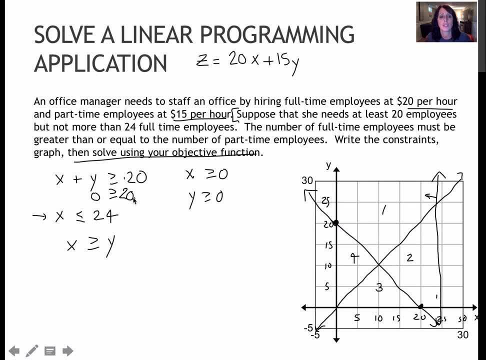 0 is greater than or equal to 20.. False, So that means it's not 3 or 4. It's 1 or 2. Using a test point here, I'm going to say: choose 0, 10.. 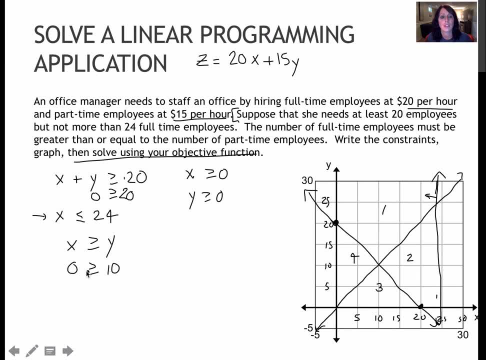 So 0 for x, 10 for y, 0, 10 would be false, which means that this line should not be shaded in this direction. So it's either basically 2 or 3.. Now, when I did this test point, 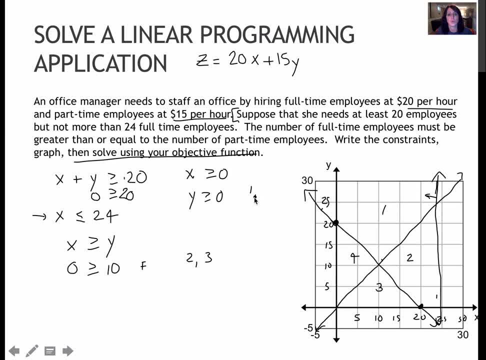 I found that it had to be 1 or 2.. So if it's 1 or 2, or 2 or 3, obviously 2 would be the little region I'm looking for. Now I am trying to find those points, the corner points. 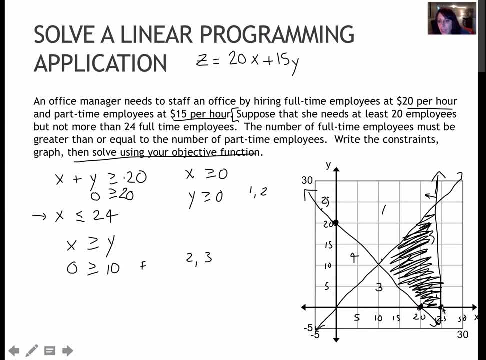 And so the corner points would be anywhere that there is a corner. And if I'm not sure if there's a corner there, then I know that I've got to do some mathematical work. So this point is clearly 10, 10.. 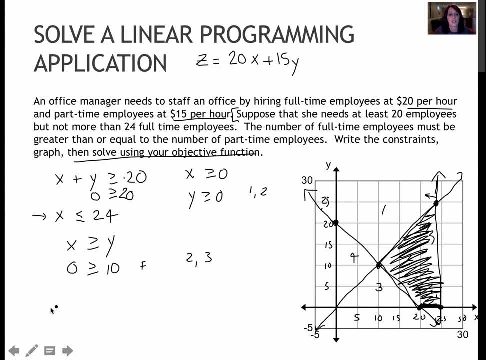 It's pretty clear that that goes through. So 10, 10 is a point. This point is 20, 0.. This point is 24.. And this point is 24 comma something And obviously, knowing that it goes through this, 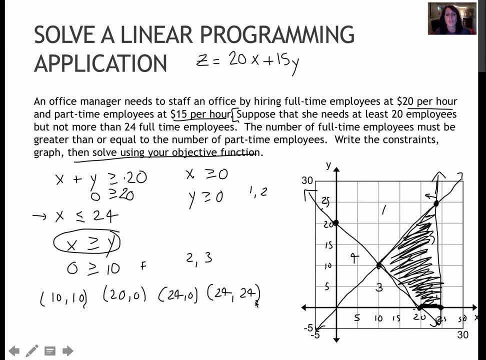 it must be the point 24, comma 24.. So this one wasn't so bad. I need all four of those points. And why do I need those points? Because I'm now going to use them in this objective function. Now, this is a cost function. 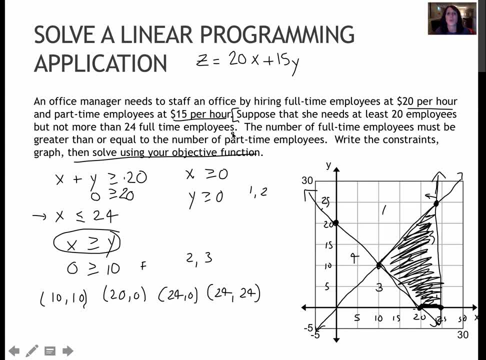 So would I want to minimize cost or maximize cost? Obviously I want to minimize the cost. So in plugging in 10,, 10,, I'm going to find out what z- or sometimes you'll see it written as z, x, y- is. 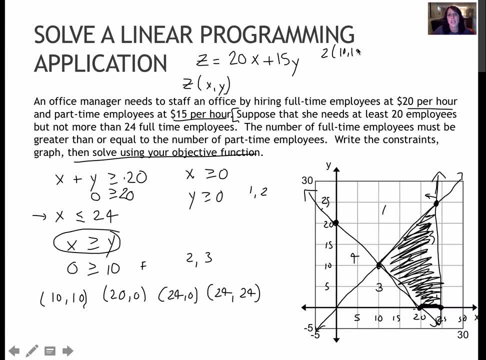 So if I find z of 10 comma 10, that means 20 times 10 or 200, plus 15 times 10 or 150.. So that's 350.. If I find z of 20 comma 0, I get 20,. 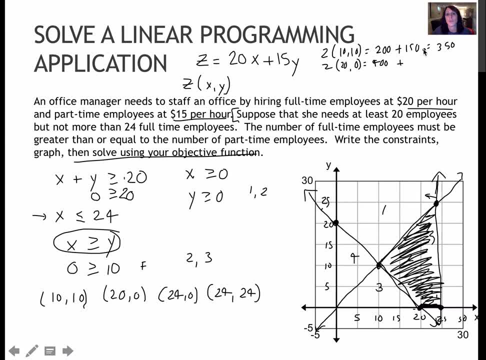 times 20,, which is 400, plus 150, or 15 times 0,, which is 0.. If I find z of 24, 0, I don't like where this one's going anyway. So that's 480 plus 0. 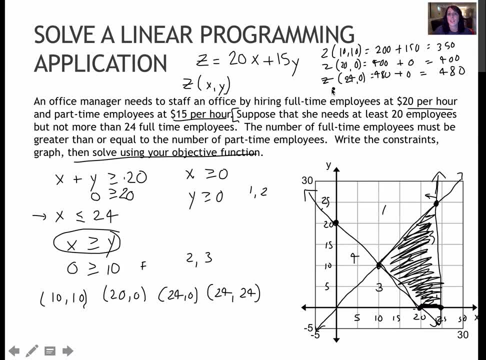 That's an increased cost. I don't want that. Last one is 24 comma 24, which is 480 plus 360 for a total of 840.. Now I know I'm trying to minimize cost, So what's the cheapest cost? 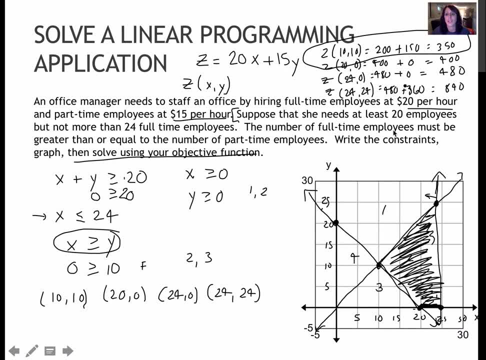 The cheapest cost is that I have 10 of each. So this point, 10, 10 would be minimizing the cost by having 20 employees would be 10, at least 20 employees. So I've got that. So 10 that are full-time and 10 that are part-time. 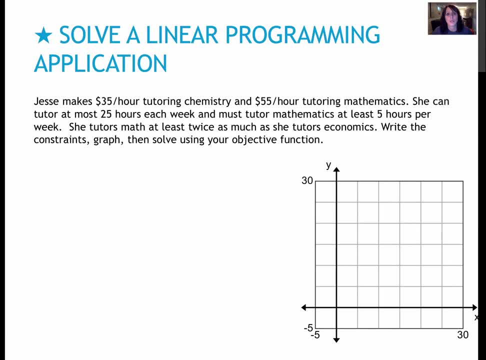 This application has to do with Jessie and her tutoring, So press pause, try this question and then press play to check your work Again. previously we did write our objective function, which was z of x. y equals 35x plus 55y. 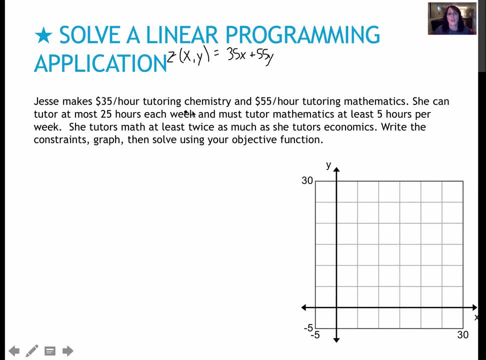 And then we have all of this other information here. So we need to write the constraints, And, of course, the two constraints that are easier: x is greater than or equal to 0,. y is greater than or equal to 0, which means that it's here, in the first quadrant. 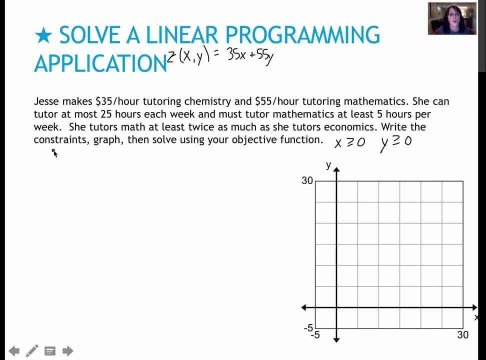 She can tutor at most 25 hours each week. So hours tutoring x or y, which is chemistry or math, less than or equal to 25.. Must tutor mathematics at least five hours per week. So math, which was y, has to be greater than or equal to five. 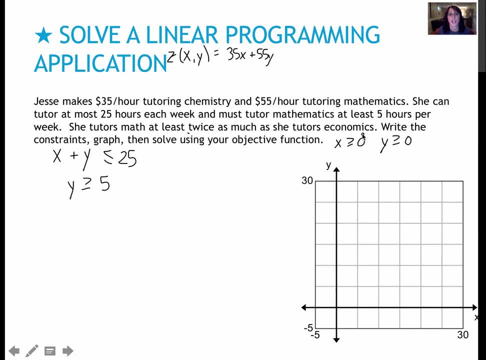 She tutors math at least twice as much as she tutors economics, And- why not? She gets paid more for it. So y is greater than or equal to 2x, And it looks like that's it. So I've got my two constraints here. 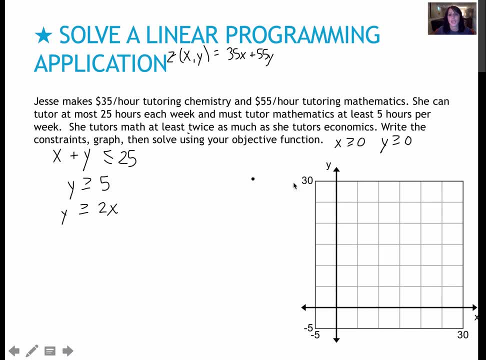 which are pretty straightforward, And then these, so this would be going through at 25 and 25.. And a solid line. I'm not going to worry about shading quite yet. This one y is greater than or equal to five. So y is five is right here. 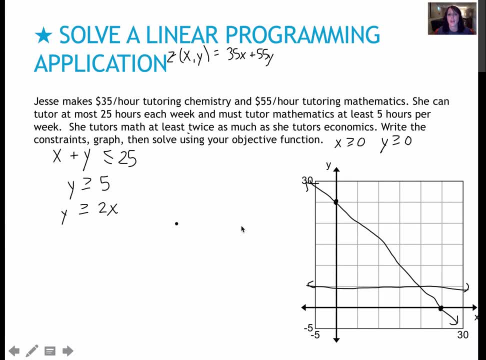 And then y is greater than or equal to 2x, which would go through at 0, 0. And then go up two over one, up two over one, et cetera, And a nice straight line there. So now let's talk about where to shade. 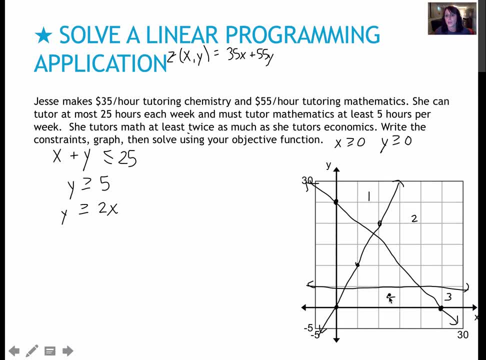 I've got one, two, three, four, five, six, seven, Seven little spaces that could be shaded. Looking at x plus y is less than or equal to 25.. That's this line, plugging in 0, 0.. 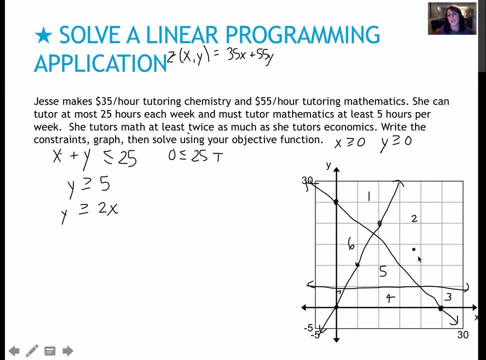 I get zero is less than or equal to 25, which is true. That means six, five, four or seven. Those are my possibilities. One can't be it, Two can't be it, Three can't be it. It's on the wrong side of that line. 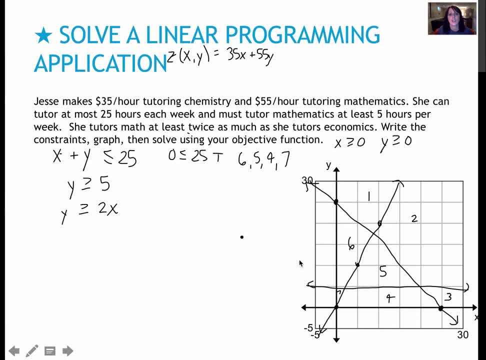 Let's try this one: Y is greater than or equal to five, Obviously greater than. if I plugged in zero, I have zero is greater than or equal to five, which is false. So this should not be shaded towards 0, 0.. 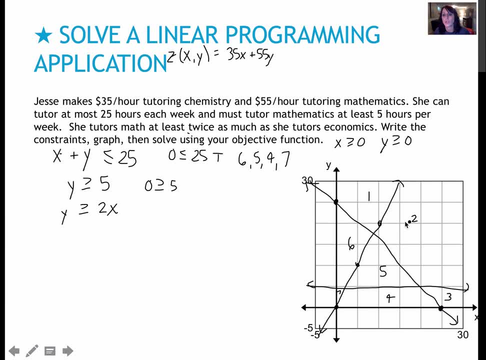 So it should be shaded above that line, which is one, two, five or six. One didn't happen here, so it can't be one. Two didn't happen here, so it can't be two. So it's either five or six, one of those two. 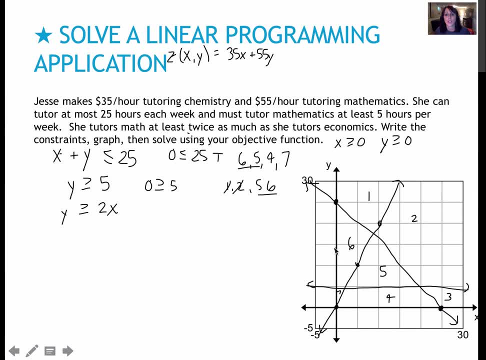 Using this one. obviously I can't use 0, 0. I could use say 0, 10, as a test point, 10 for Y, 0 for X, 0, 10 gives me 10 is greater than or equal to zero. 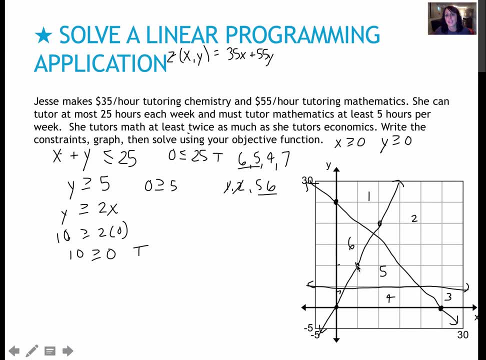 Last time I checked that was true. So that means this line should be shaded to the left, which is one or six, which of course means that it must be six because that's the only one that works. So here's my little shaded region right in here. 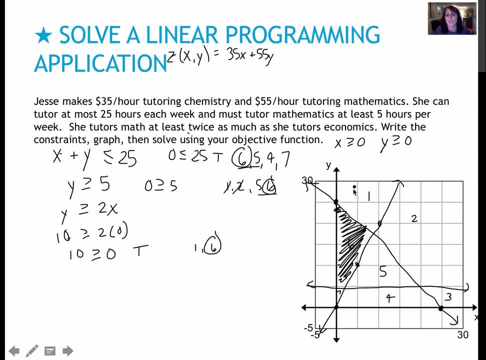 I need to find all of those corner points to plug in. so I'm gonna go ahead and do that. I'm gonna go ahead and do that. I'm gonna go ahead and plug into my objective function. This point, pretty easy, is 0, 25.. 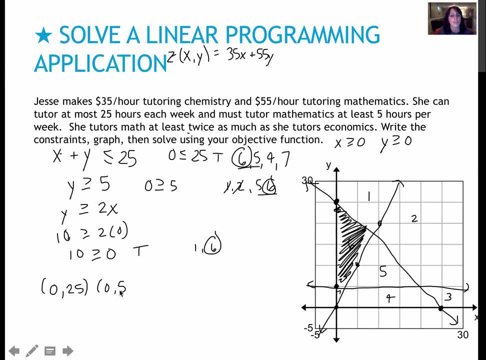 This point right here is 0, 5.. I've got this cross point right here. I have no idea what that is, and I've got this cross point right here and I don't know what that is either, So I'm gonna have to find two more points. 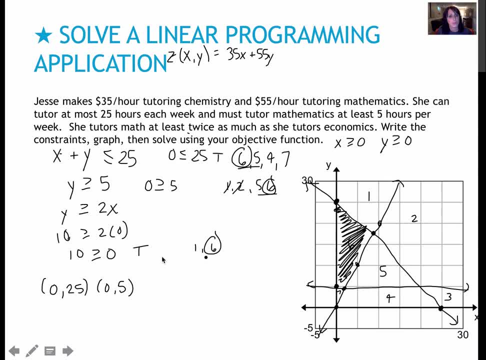 This one goes through at. This one goes through at: Y is greater than or equal to five, and this equation, which is Y is greater than or equal to two X. So I would say let's set two X equal to five. 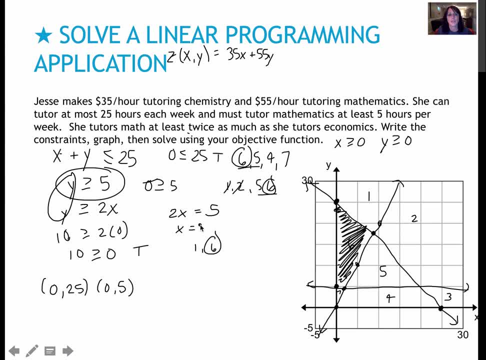 using substitution. So X must be 2.5, and of course Y would be five. So the point 2.5 comma five would be a point. How did I know that? Because obviously this is on the line right. 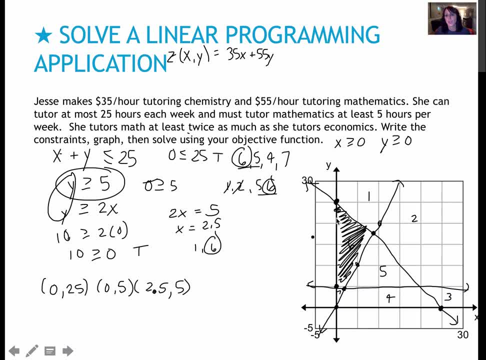 Line Y equals five, So 2.55 is another point. This point that is floating out here in the middle is where this line crosses this line. So now I have to solve using substitution there, So X plus Y, which is two X. 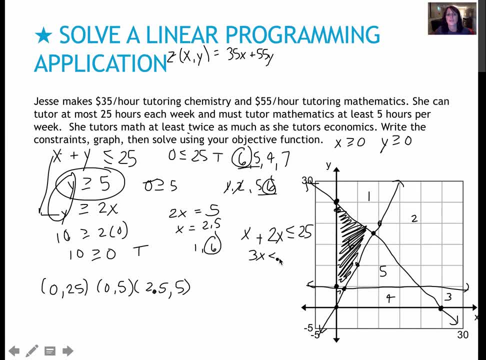 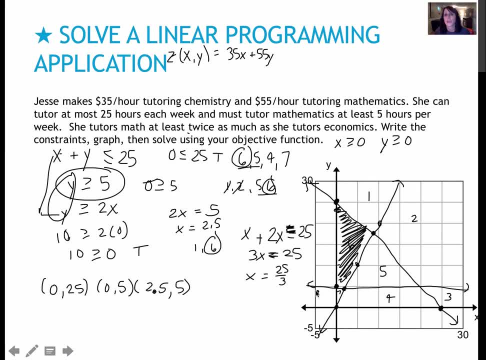 Three, X is 25, so X is 25 thirds. You can, of course, turn that into a mixed number if you would like eight and a third, which makes sense. Eight and a third would be somewhere in there. To find the Y value, I'd have to plug it back in. 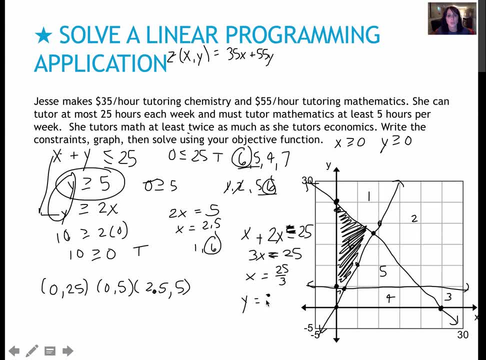 to either of those equations. So I would probably use: Y equals two times 25 thirds, which means Y is 50 thirds. So 25 thirds comma 50 thirds. So 25 thirds comma 50 thirds. So 25 thirds comma 50 thirds. 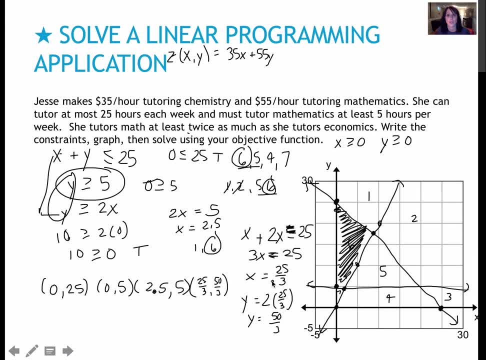 Which are decimals, And I'll probably just have to use them as decimals when I plug them in up here. So again, this is me trying. well, Jessie, trying to make money. So last time we tried to minimize, This time, obviously, we're going to maximize. 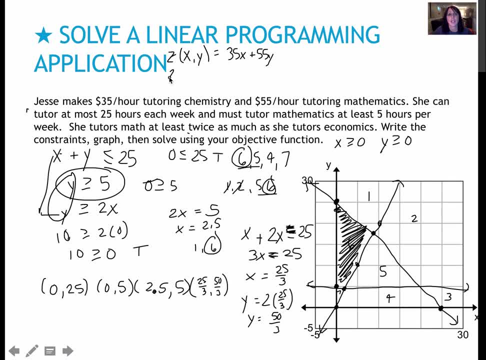 because we want to maximize our profit. So if I plug in 0, 25, which is this point right here, I get 35 times 0, plus 25, 25. Which will give me minus half of 0. КП. //. The answer is K. 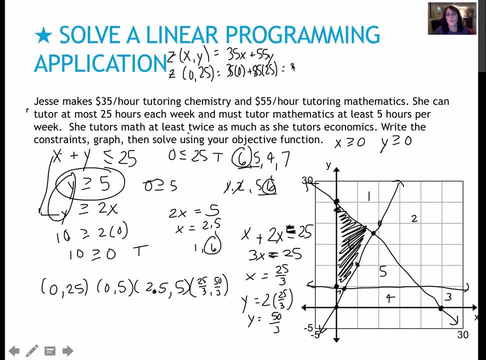 55 times 25,, which is 1,375.. Not bad. Next, I would say 0 comma 5.. I already know this one's not going to be awesome: 35 times 0 plus 55 times 5,, which would of course be. 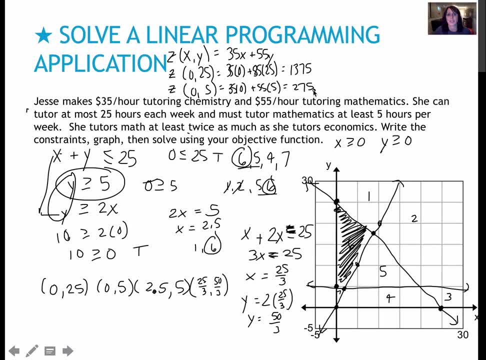 275, which that's not going to be the maximization. Let's plug in 2.5 comma 5.. So I have 35 times 2.5 plus 55 times 5.. That gives me 362.50.. Again, not maximized. And my last one.